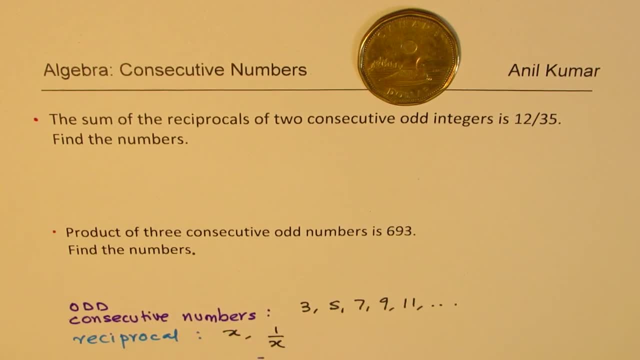 then the reciprocal is 1 over x, right? So these are reciprocal numbers, right? So, for example, if you're talking about these odd numbers, the reciprocal numbers will be 1 over 3, 1 over 5,. 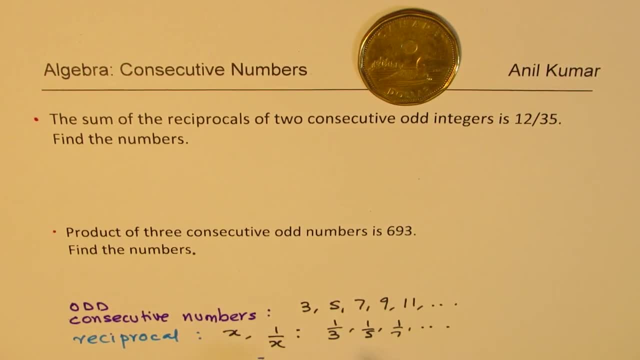 1 over 7, and so on. You get the idea right. So these are reciprocals of the consecutive numbers, odd consecutive numbers. Perfect Now, once we understand this strategy, now look into the solution of these questions. The first one here is the sum of reciprocals of two consecutive 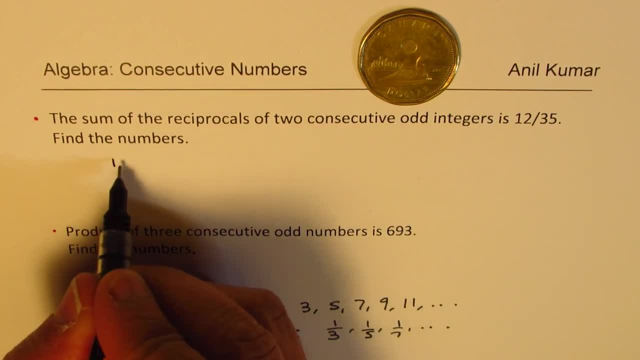 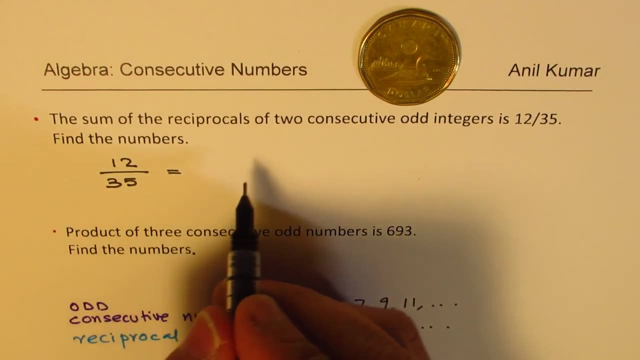 odd integers is 12 over 35. So let me write down 12 over 35.. Now 35 could be written as product of what 7 times 5, right? So we could write this as 12 over 7 times 5, and that gives. 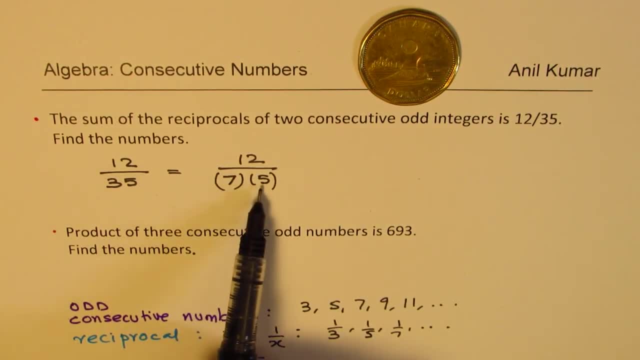 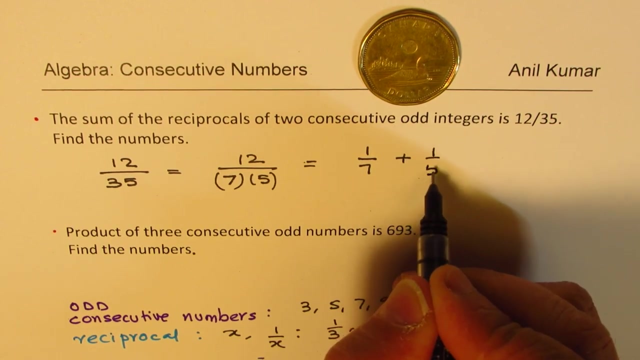 me 35. And we also understand that 7 and 5 are consecutive odd integers. So if you have to look into this, you could think like this that we are talking about something which is kind of 1 over 7 plus 1 over 5, right, So that actually gives you 12,. 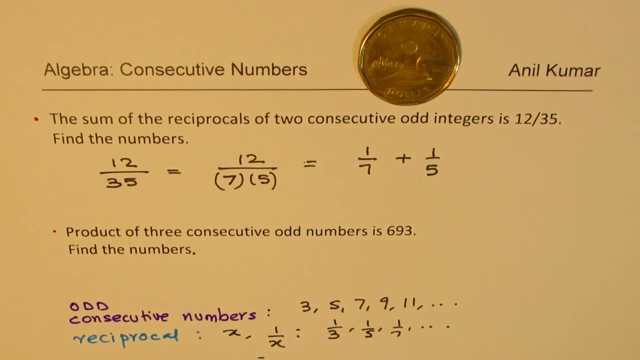 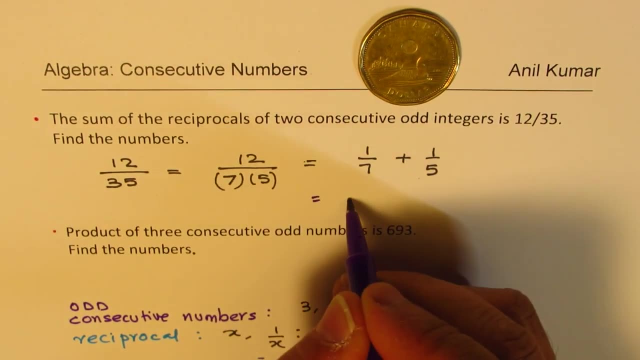 5 times 1 and 7 times 1, right Cross multiply And what you get here is, if you want to work on this, 1 over 7 plus 1 over 5, common denominator is 35. And what we get here is 5 plus 7,, which is: 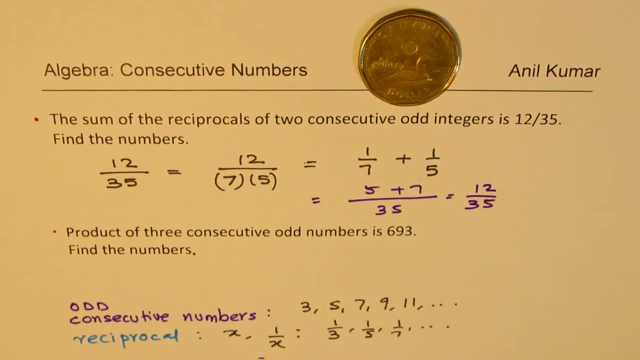 12 over 35. And therefore, what is the answer? Well, so we get our answer here, and the answer is: the question is the sum of the reciprocals of two consecutive integers? is this: Find the numbers. We have to provide the numbers. So the numbers are 5 and 7, right, So that becomes our. 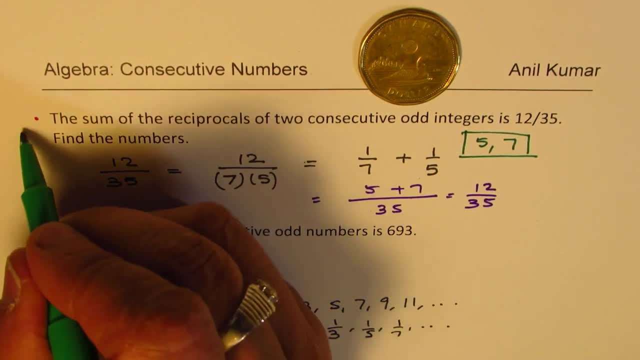 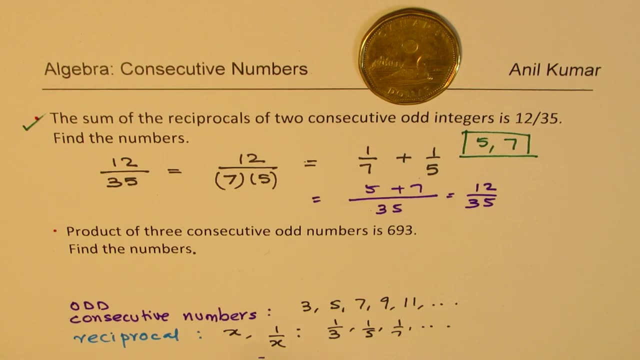 answer. Is that clear to you? So that is how we are going to do the first question. Now let us look into the second question. So let us look into the third question. So let us look into the solution of the second question. It is product of three consecutive odd integers. So in this, 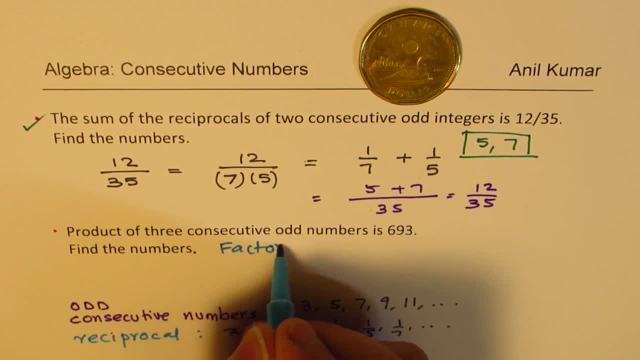 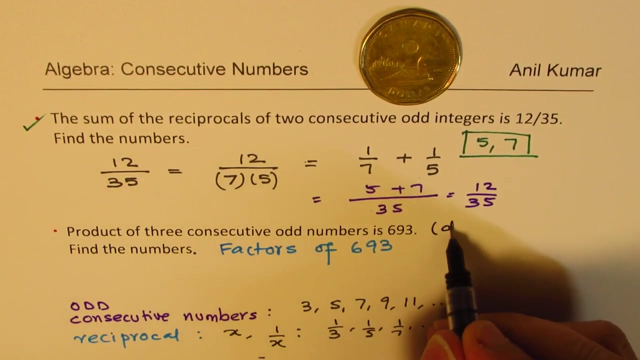 my strategy will be to find factors right. So find factors of 6,, 9,, 3.. How do you find factors of 6,, 9,, 3?? Well, 6,, 9,, 3, 6 plus 3 is 9, and that is 9.. So it is divisible by.